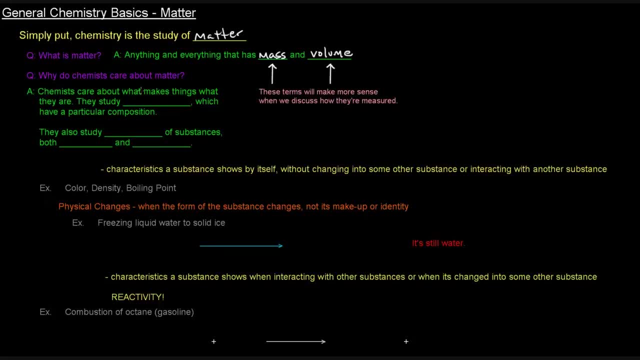 But now, why do chemists care about matter? Because it matters. Chemists care about what things, or what makes things what they are. They study substances, which are things, Things that have a particular composition or a particular makeup. We'll talk more about the definition of substances and what kind of classifies or is classified as a substance. We'll talk about that later. But they also study the properties, the properties of substances, And these properties include both physical and chemical properties. So what is a physical property and what is a chemical property? 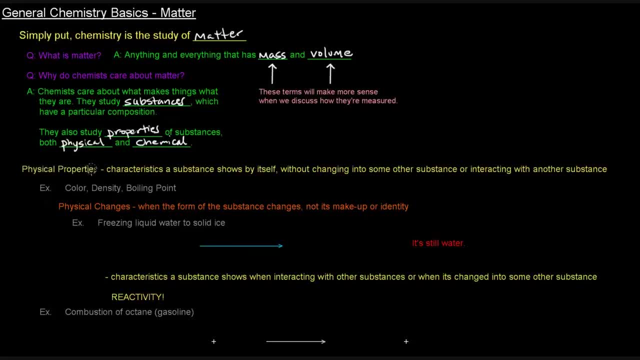 Well, let's start with physical properties. Physical properties are characteristics a substance shows by itself, without changing into some other substance or interacting with another substance. Okay, so this is pretty important. One really really important part of this definition is the by itself, bit By itself and without changing. Those are important parts. 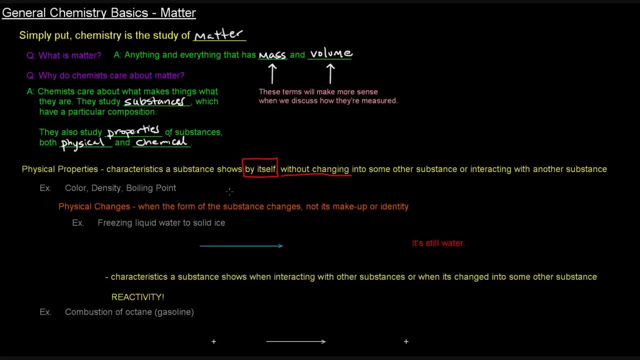 So physical properties are characteristics of a substance that that substance shows. So physical properties are characteristics of a substance that that substance shows by itself and it's not changing into something else or interacting with something else or some other substance. So some examples are color or density, boiling point, even melting point. 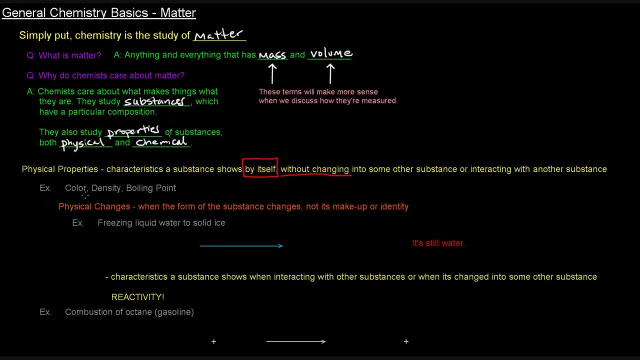 Color, for instance, like water, Water is a clear. it's clear right when it's a liquid And also when it's solid as well. That's a physical property. That's a physical property. Water's density at 25 degrees Celsius and one atmospheric pressure is one gram per milliliter. 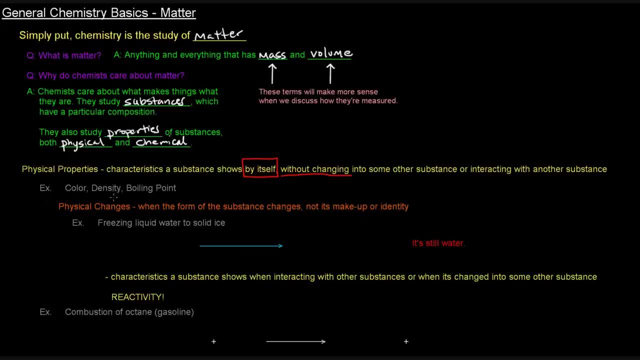 That can vary slightly, But the point is these are physical properties, These are things that these are characteristics of a substance that are independent of another substance interacting with this particular substance. I use the word substance a lot there, but hopefully I can kind of explain this with an example. 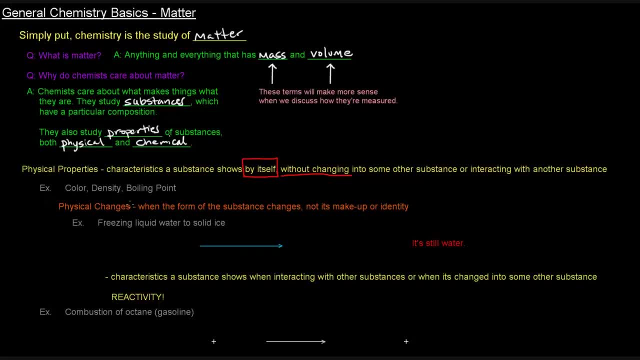 With an example of a physical change specifically. So physical changes are changes that occur when the form of the substance changes, not its makeup or identity. So this is a this is an important part: The form changes, not the identity. Ok, 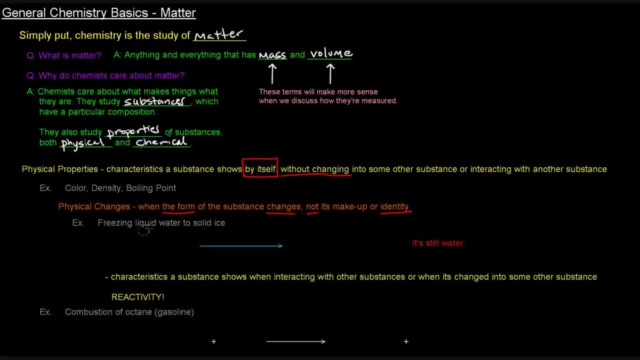 So let's think about the example of freezing liquid water into solid ice. So a lot of people know that H2O is the chemical formula for water. And this little, this little- in parentheses, here is a little cursive L. 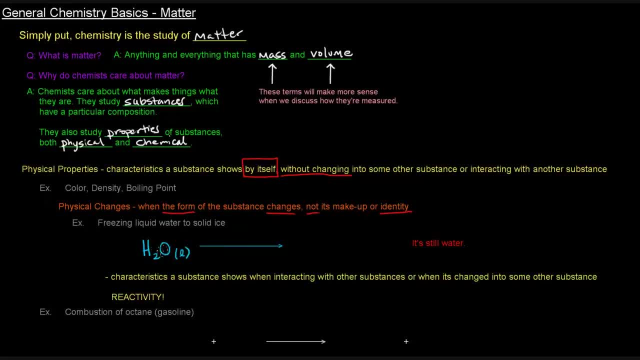 L, which means liquid. we'll talk more about that later. but water in liquid form can turn into water in the solid form, And that's what happens when we're taking liquid water and turning it into solid ice. Isn't it still water? Yeah, it's still water. It hasn't changed. 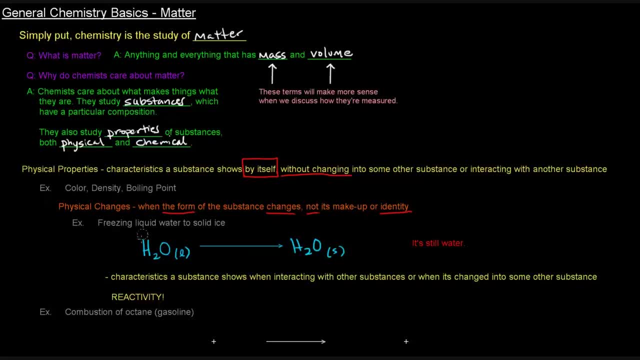 its identity. That is a physical change. So you know water being a liquid at room temperature and a solid at really cold temperatures, specifically colder than 0 degrees Celsius or 32 degrees Fahrenheit or 273 Kelvin. that is a physical property, whether it's a liquid or a solid. 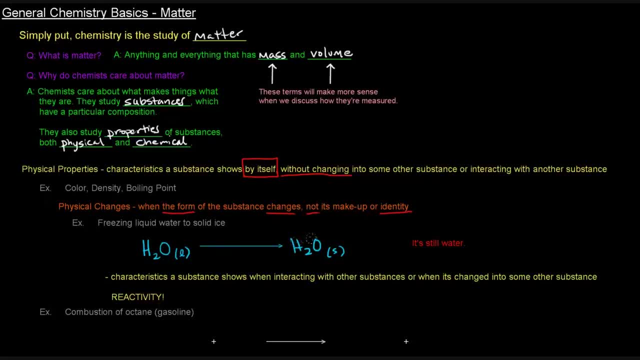 And this is a physical change, changing from liquid to solid. Its identity hasn't changed: It's still water, And that's what I meant by by itself, without changing into some other substance. It's still the same thing. Now let's talk about chemical properties, Chemical. 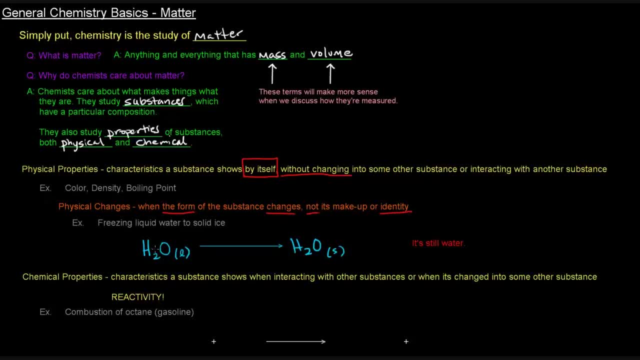 properties, as you might imagine, their characteristics a substance shows when an individual is interacting with other substances. So that's that's the important part of this definition: interacting with other substances or when it's changed- That's also a really important term- into some other substance. So really, chemical properties basically describe the reactivity. 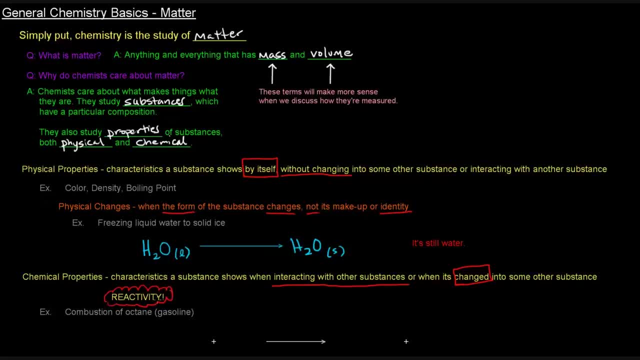 of a certain substance, And there are of course, chemical changes. as opposed to physical changes And chemical changes, chemical changes have another name, Really, they're called chemical reactions, And so we're talking about when one substance interacts with another substance and changes to some other. 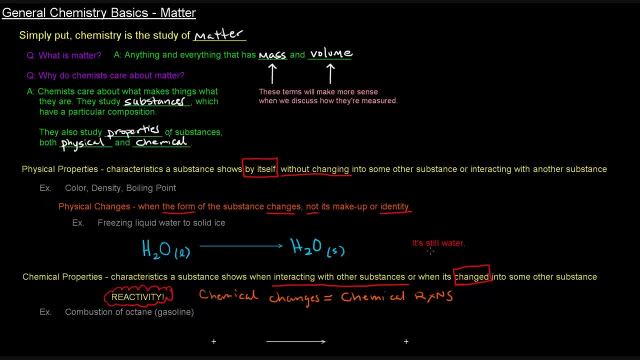 substance. It doesn't even have to interact with something necessarily as long as it changes its substance, But I think pretty much, pretty much all the time it's interacting with something else. In fact I have an example here of a chemical reaction, Um. 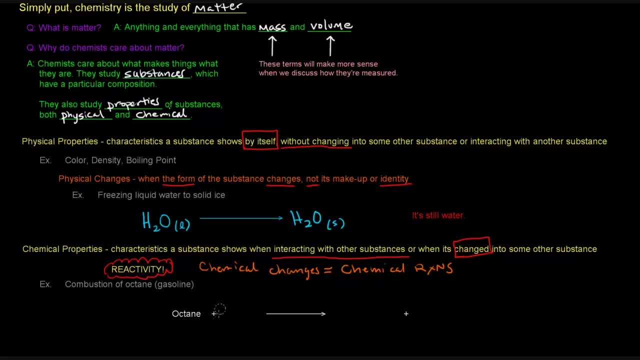 the example is the combustion of octane, which is gasoline. So if you take octane and oxygen um and you put them together, add a little bit of heat, what happens is that we change these two initial substances that we start with. 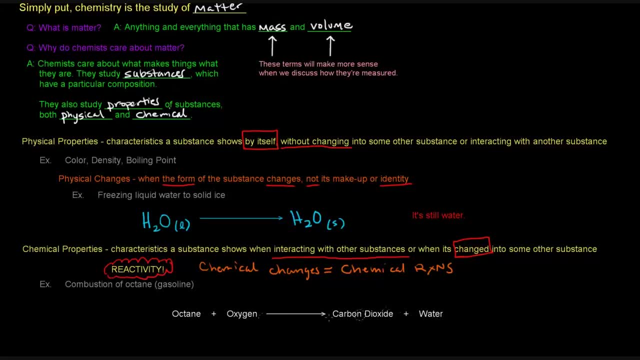 octane and oxygen. we change them into carbon dioxide and water. That's a chemical reaction. So it's a chemical property of octane, which is the chemical for that is used for gasoline, to power up and so on, to power our cars and even lawnmowers and stuff um. but octane has a certain level of reactivity. 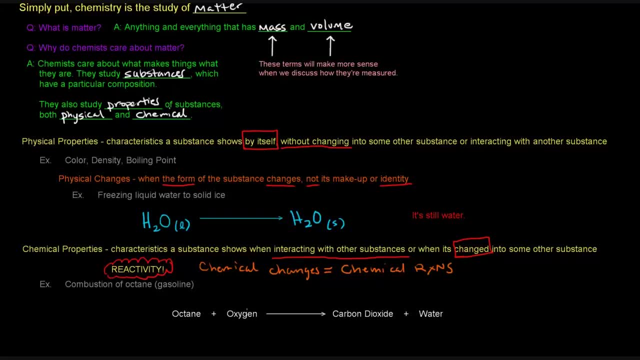 with oxygen and, if there's enough heat, it can cause this to basically explode, um, and create carbon dioxide and water, and this, of course, this is a reaction that releases energy, which is another thing that we'll talk about later, but the point is that we start off. we start off with octane. 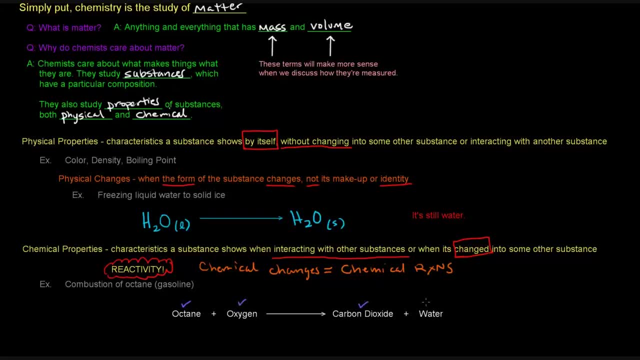 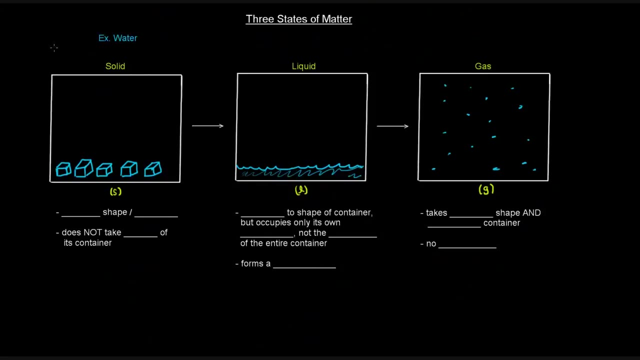 and oxygen and those things are changed into carbon dioxide and water. we no longer have octane and oxygen. so it's a chemical property of octane the way it reacts with oxygen. next up, the three states of matter. so you may or may not have already known this, but the three. 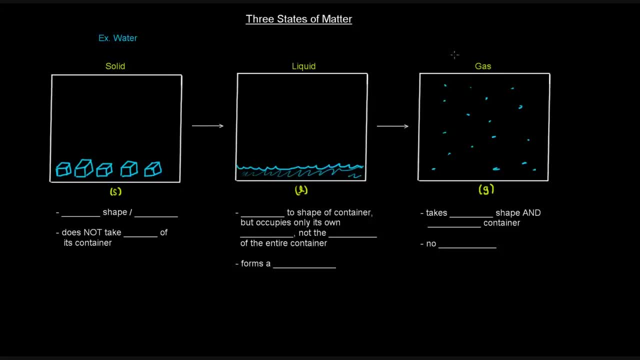 states of matter are solid, liquid and gas um, and i think one of the simplest ways to kind of understand this is really to just talk about it in terms of an example, and the simplest example is is water. so we know that water? um can increase the amount of oxygen that we're producing. so we know that water can increase the amount of. 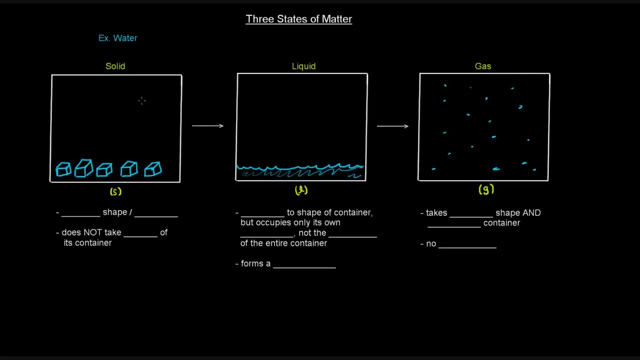 oxygen that we're producing. so we know that water can increase the amount of oxygen that we're producing and of course that can also exist as solid, uh, solid that we call ice, right um. and of course it can exist the liquid that we drink, and it can also exist as a gas, which is we call water vapor. so 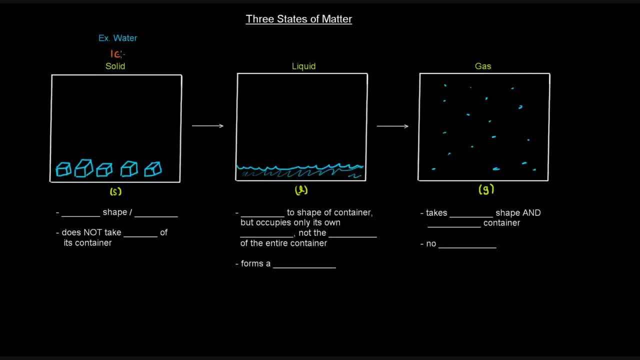 i'll put all those little terms here as well. so here we got ice, solid liquid water, and then, uh, water vapor is the gas. okay, so what are some of the characteristics of, you know, solids and liquids and gas? what defines them? well, solids, solids have a fixed shape. they have a fixed shape and volume. they have a fixed shape and volume. 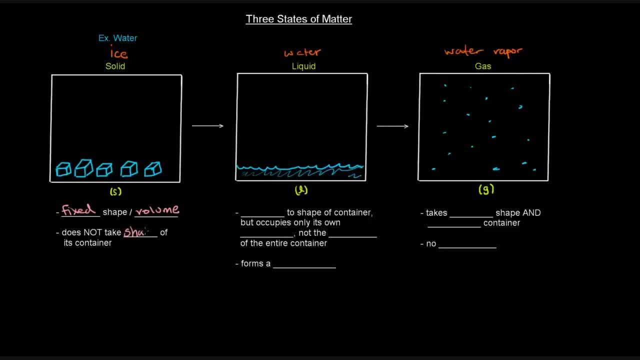 they do not take the shape of their container. so if you put ice into like a beaker or a bucket, it's only going to take up as much space as it takes up as it's, it's in its ice form. it's not going to take the volume of the 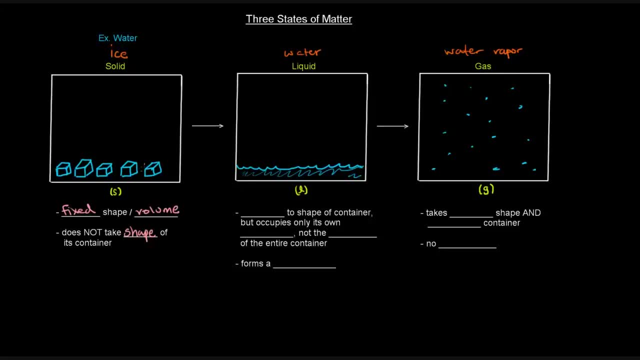 container doesn't flow at all. it's very fixed and definite shape and volume. liquids, however liquids they they kind of flow right, they conform to the shape of their container, but it occupies only its own volume, not the volume of the entire container, in the way that a gas does, which we'll get to in just a second. 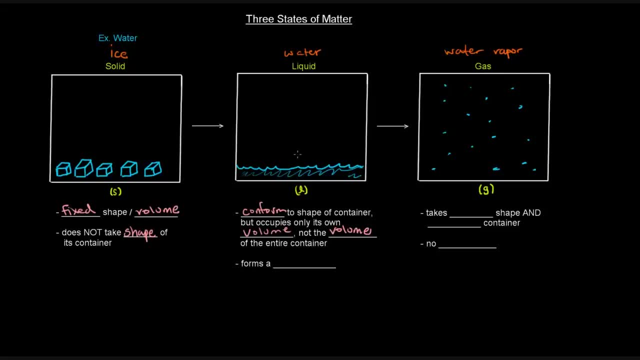 so if you put a liquid into a cup or a beaker- liquid water specifically- and you kind of, you know, swish around the, the cup, the, the, the water will kind of, or the liquid will kind of, you know, go back and forth and kind of adhere to the, the, 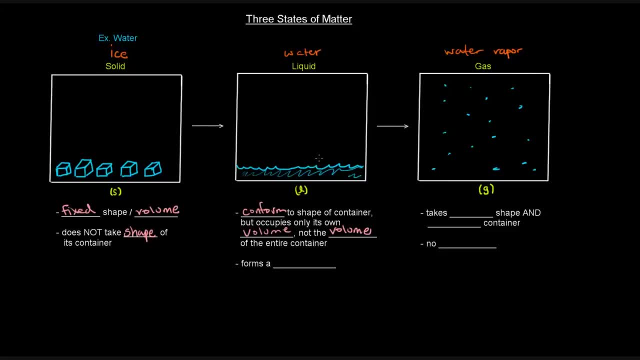 shape of the container. if you have a round glass, it'll take the shape of a round glass but it doesn't take the entire volume of the the container. it doesn't take up the entire space of the container, it only takes up its own volume conforms to the shape of the container only to a certain extent. 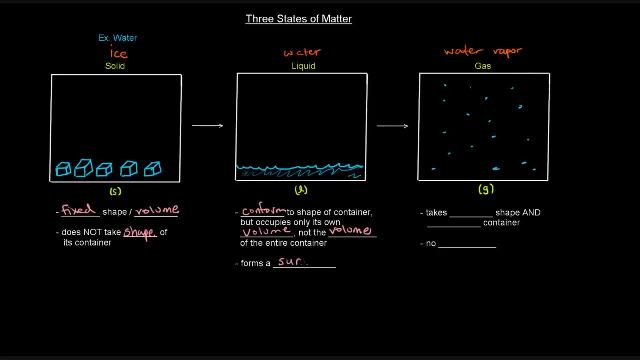 Another thing about liquids is that they form what's called a surface right So you can have when you once you know, at the top of its it takes the volume of its, excuse me, it takes the shape of its container. 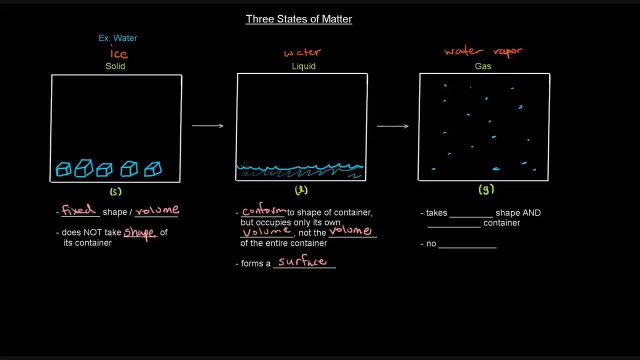 to a certain extent, but it does have a surface that you can kind of clearly see. Gases, however, they take the entire surface, shape and volume of their containers. They fill the entire container. So if you have a small cup and you, you know, have it shut. 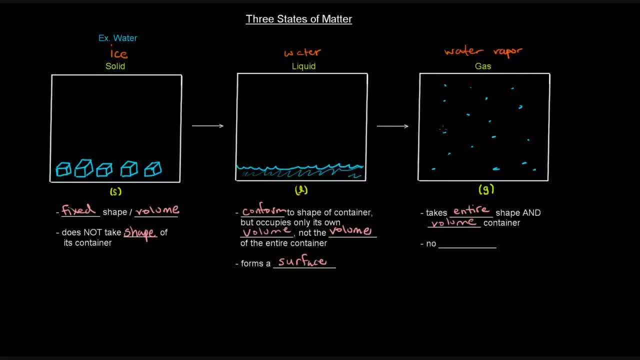 and you initially have some liquid in there, some liquid water, and you boil it and it all becomes gaseous water vapor. that water vapor will take up the entire volume of the container And it of course takes the shape as well, because it fills the entire space of its container. 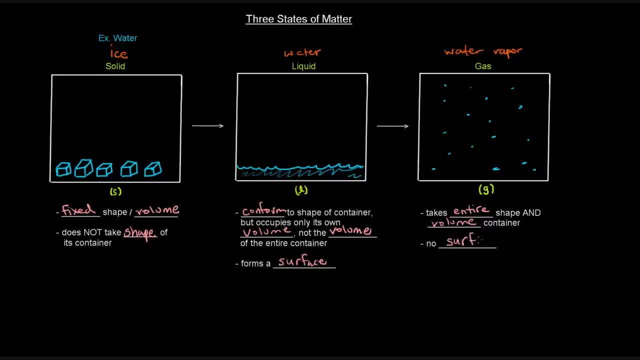 And, of course, because of this, it'll have no surface. So these are. These are just some details. I don't want to go into too many because this is just a video about the basics, But I hope that video was helpful.